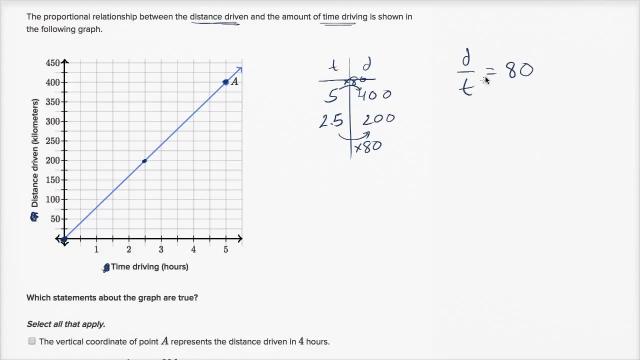 that we're dealing with a rate. Distance is in kilometers, time is in hours. 80 kilometers per hour. This is the rate at which we are driving. We are going at this speed: 80 kilometers per hour. This is also the proportionality constant. 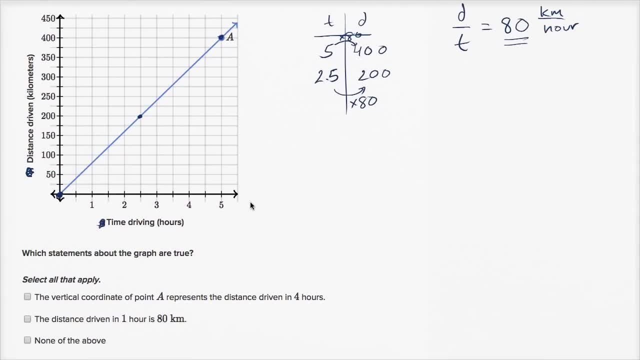 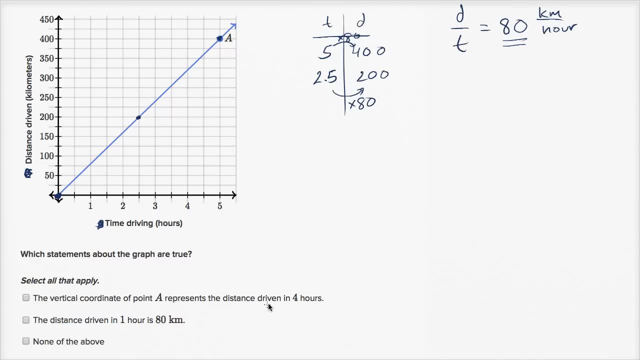 Well, anyway, with all of that out of the way, let's actually answer the questions. Which statements about the graph are true? Select all that apply. The vertical coordinate of Point A represents the distance driven in four hours. The vertical coordinate of Point A. 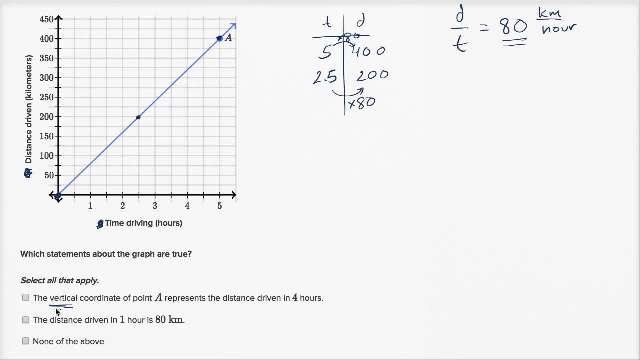 represents the distance driven in four hours. The vertical coordinate of Point A represents the distance driven in four hours. the vertical coordinate, the vertical coordinate. So point A is at the coordinate five comma 400.. Now the vertical coordinate tells us how high to go up. 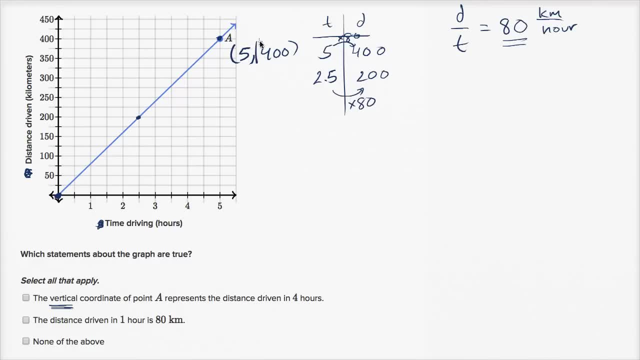 how far to move in the vertical direction. That's going to be the second coordinate right over here. So this is the vertical coordinate. So this right over here tells us the distance we've driven in four hours. So yes, the vertical coordinate of point A. 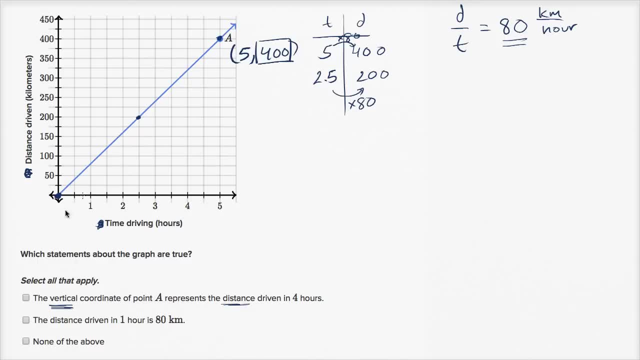 represents the distance driven in four hours. We've driven 400 kilometers, so I like that one. I'll check that one. The distance driven in one hour is 80 kilometers. The distance driven in one hour is 80 kilometers. Well, when you just try to eyeball it. 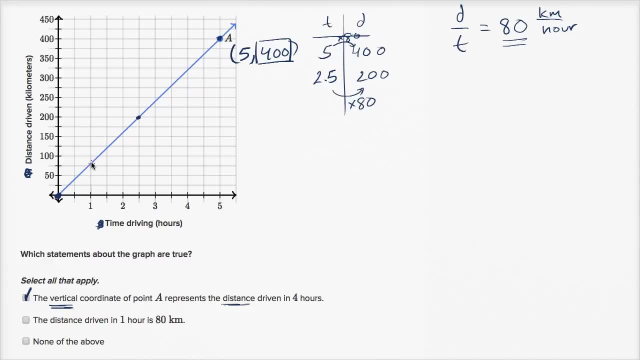 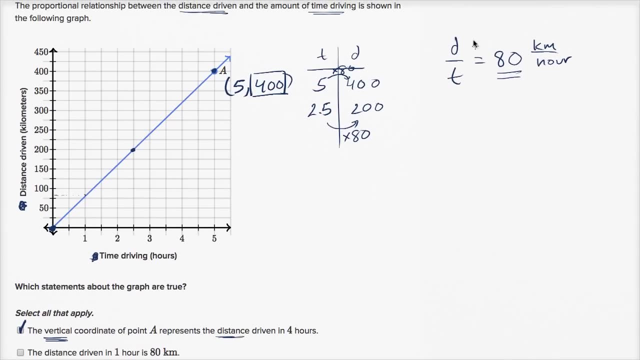 off of the graph here. see, after one hour it looks like it's a little bit more than 75, so, yeah, 80 seems like a reasonable one. But we see it even more clearly when we look at the calculation that we did. 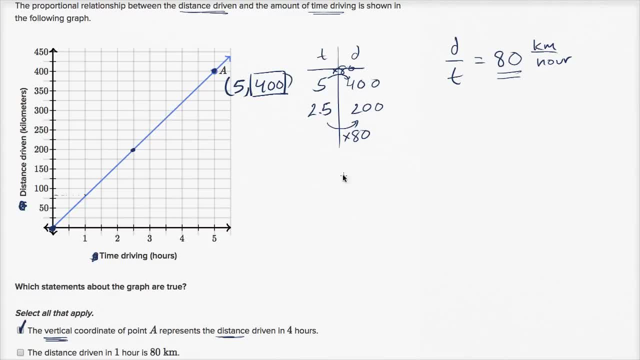 If you take a distance, if you take a distance, any one of these distance- 400 kilometers, 400 kilometers over five hours- tells you that your rate is 80 kilometers per hour And you know this is going to happen for any point on this line. 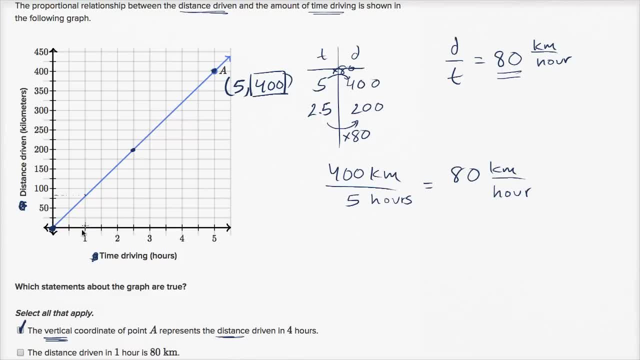 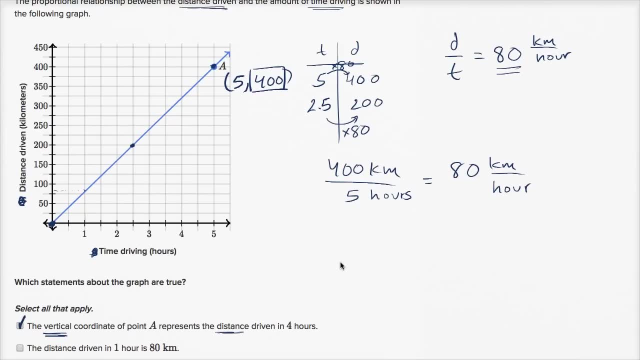 They tell us it's a proportional relationship and we can tell visually it's a proportional relationship. It goes to the origin and it is a line. So the distance traveled in one hour is going to be 80 kilometers. It is going to be 80 kilometers. 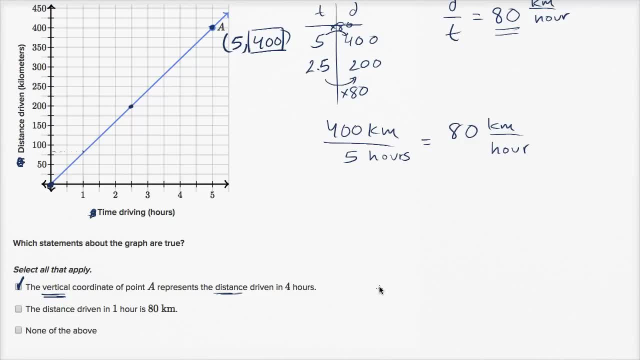 because we're going 80 kilometers per hour. So in one hour we're going to go 80 kilometers, So I like that choice as well. Of course, I won't pick one of the above because I found two choices that I liked. 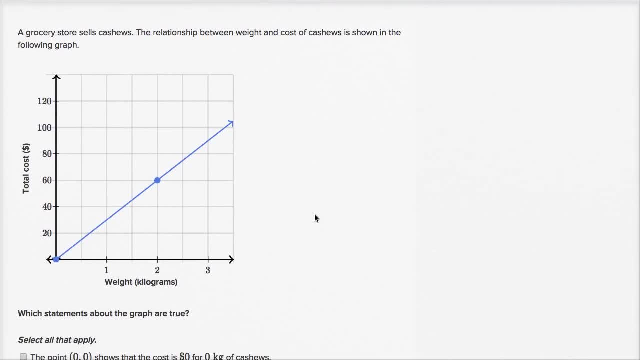 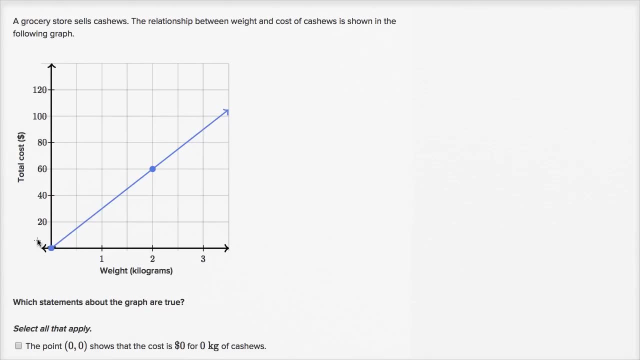 Let's do another one of these. This is fun. A grocery store sells cashews. The relationship between weight and cost of cashews is shown in the following graph And once again we see it as a proportional relationship. It goes through the origin and it is a line. 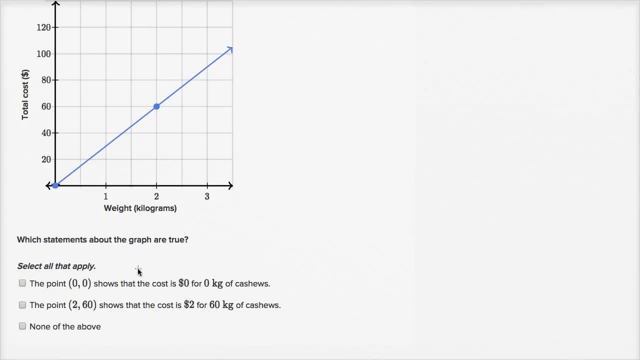 Which statements about the graph are true. Select all that apply. The point zero: zero shows the cost is zero dollars for zero kilograms of cashews. Yeah, zero kilograms of cashews, it's zero dollars. Yep, that makes sense. The point two, comma 60,. 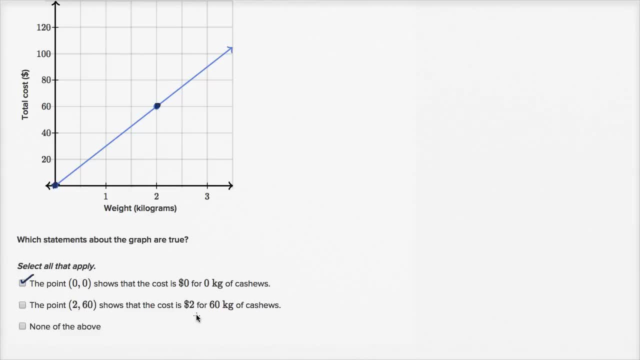 that's this point right over here- shows the cost is two dollars for 60 kilograms of cashews. The cost is two dollars for 60 kilograms of cashews. No, this is showing us that the cost is $60.. The cost is $60 for two kilograms. 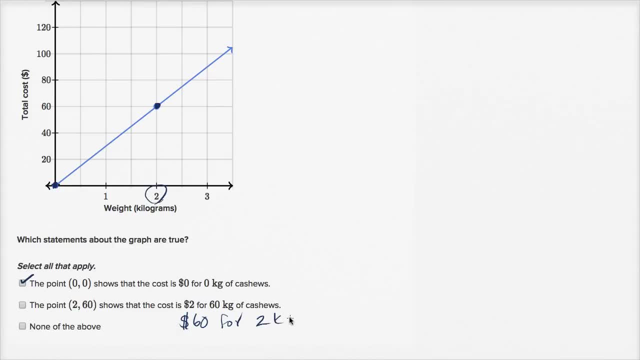 for two kilograms, for two kilograms of cashews, This axis right over here, this is weight. Actually, if you're measuring kilograms, you're really talking about mass. But anyway, I don't want to get too particular here. But this: you have a mass here of two kilograms. 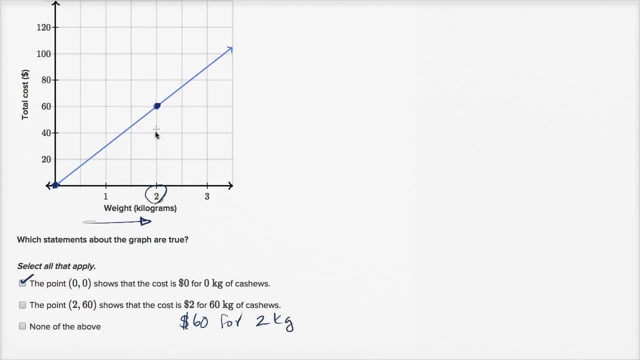 So the- I guess you could say- the horizontal coordinate tells you the mass, The vertical coordinate tells you the cost And that is 60, $60.. So it's $60 for two kilograms, Not $2 for 60 kilograms. That would be a deal. 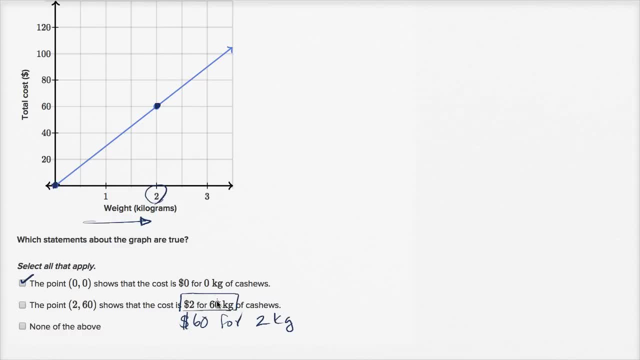 If you could get, if you could get $60 for 60 kilograms. $60 for 60 kilograms that would be a deal. But if you could get, you know, this is kind of what a medium-sized grown man would weigh: 60 kilograms. 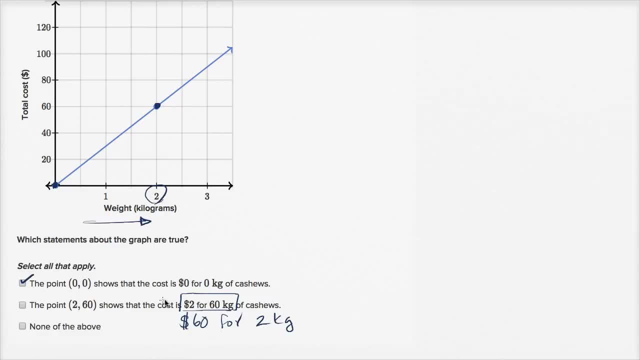 And $2 for that much, that much cashews, that would be an incredible deal. So you definitely want to rule that one out. And I'm not going to pick none of the above because I already figured out that I liked. I liked the first choice up there. 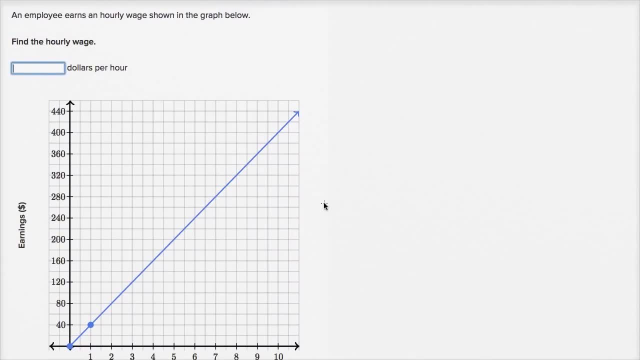 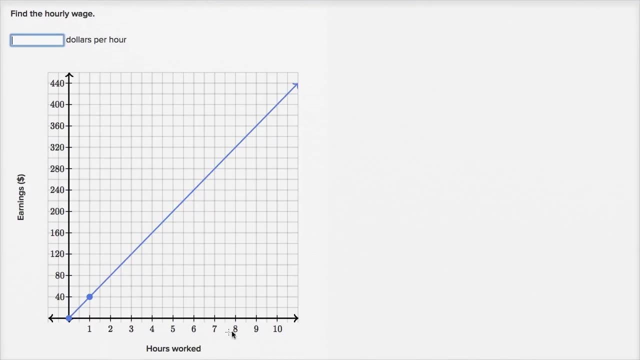 Let's just do one more, just for good measure. An employee earns an hourly wage, shown in the graph below. Find the hourly wage. So we see here in the horizontal axis we have hours worked And in the vertical axis earnings. 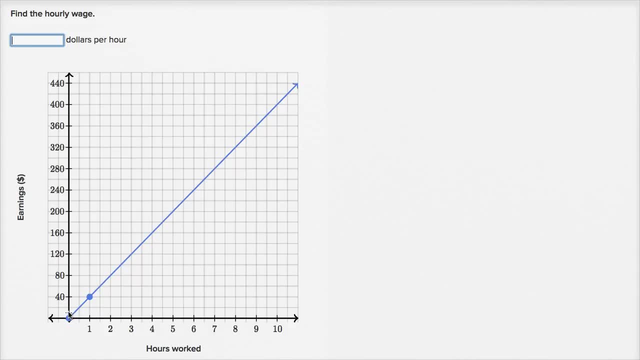 We see it's a proportional relationship That the, that the and that makes sense. The ratio between earnings and hours should always be constant. If we're earning money at a constant rate, we see it visually, we go through the origin.